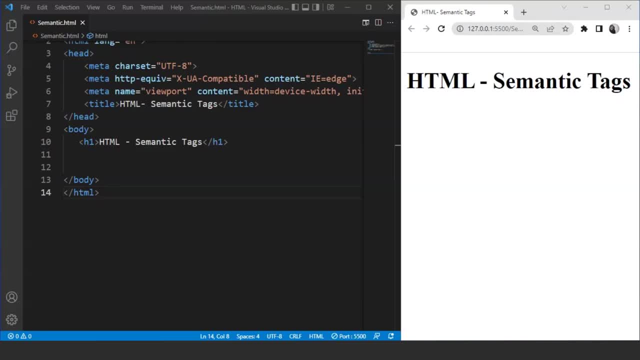 div tag in HTML. On the other hand, Semantic Tags refers to elements or tags that define their meaning to the browser and the developer. Now, for example, when we create a navigation bar for a web page, we have two options. We can either move to the body tag and we can write here div id as, let's say, nav. 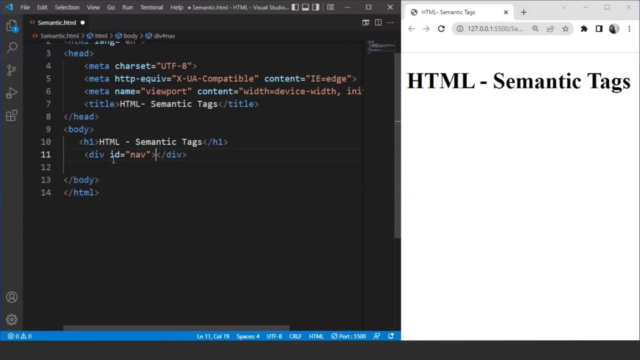 Then we have to move to the CSS file and we have to use certain properties or we have to add the data in here inside the div tag to create a particular good looking navigation bar. The div tag we use will specify only a division in the browser. 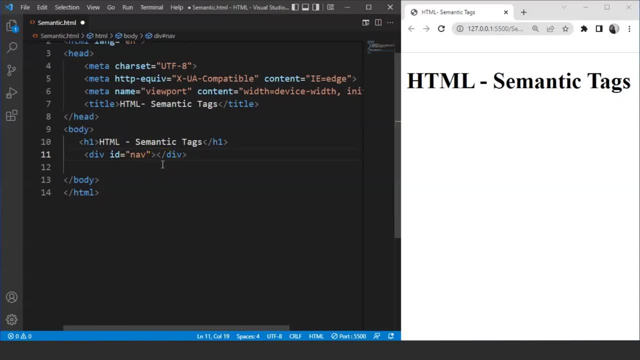 It has no meaning at all. Fine, The other way of creating this navigation bar is by using the nav element. The nav element means that anything that goes inside the body of the nav tag- So we have to write here nav, This tag specify that any content goes there inside this tag will represent the navigation. 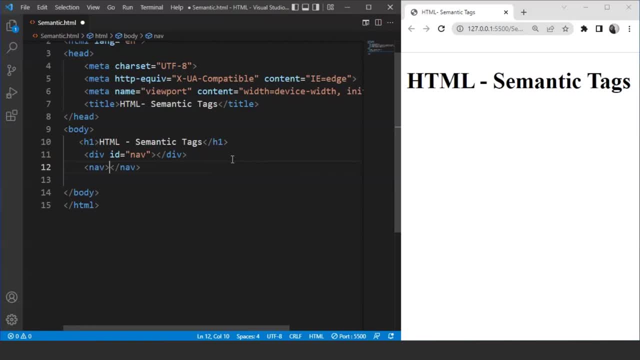 bar of our web page. Fine, So this is the difference between non-semantic tags and semantic tags. in HTML, The div tag falls under the category of non-semantic tag And the nav tag falls under the category of non-semantic tag. 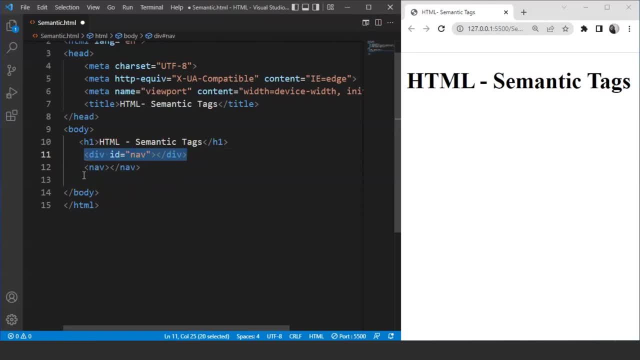 Fine. A lot of tags are present in HTML, which falls under the category of semantic tags. We have already discussed them in the previous video. So the list goes like this: We have the article tag, aside tag, Then we have details, figure, footer, header, mark, nav, section, summary and time. 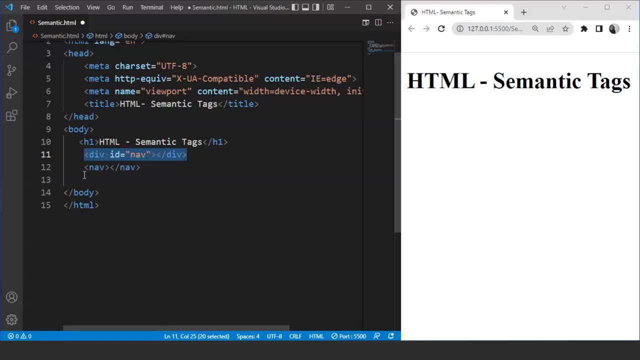 So we have already discussed most of them previously. like the article, header, figures, mark, nav, etc. The detail tag is quite interesting to go through, So let's go through this tag and we'll see its usage and syntax. Now the details tag is used along with the summary tag to create interactive widgets. 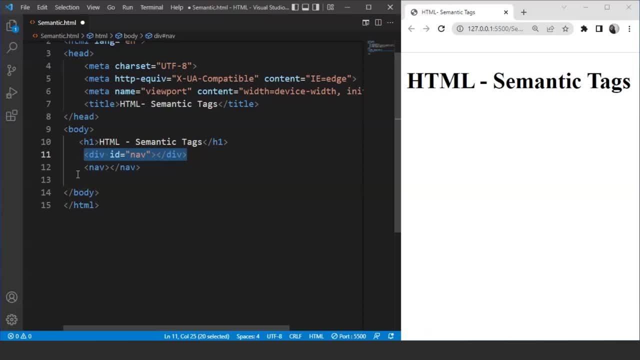 using HTML. Widgets on a web page are mainly created with the help of jQuery and jQuery UI, But HTML 5.0 also provides us a way to achieve this task. We are going to create a widget using HTML. Fine, So let's remove it from here. 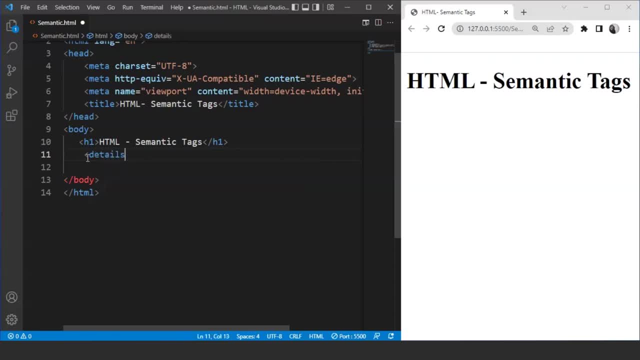 We are going to create a widget using HTML. We are going to use the details tag, So we'll write here details. This is the body of a details element. Now what we'll do is we'll use the summary tag inside, So we'll write here summary. 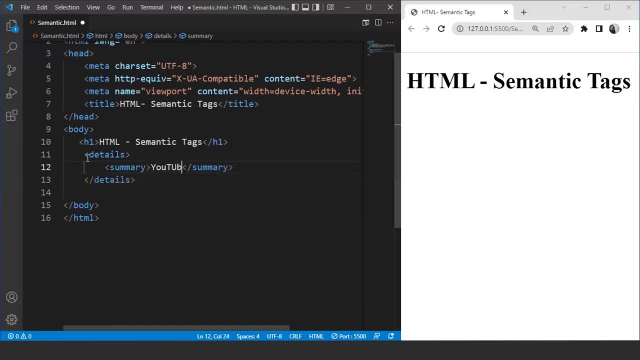 Fine, Let's write something over here. So let's say we are writing over here YouTube, And then we'll use a paragraph over here. Fine, So we'll use the tag for that. Let's say: we'll write here: go to YouTube. 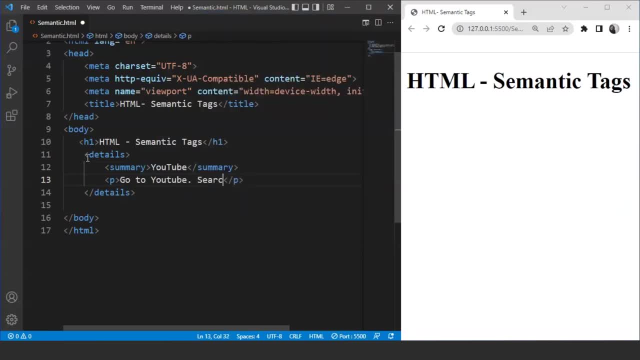 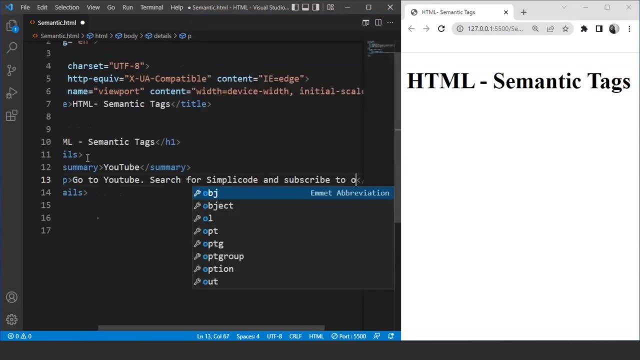 Search, Go to YouTube, Search for Simply Code and subscribe to our channel. Fine, Now, using the detail tag can make our web page more interactive for the user. It is an example of semantic tags in HTML, So the word details defines itself right. 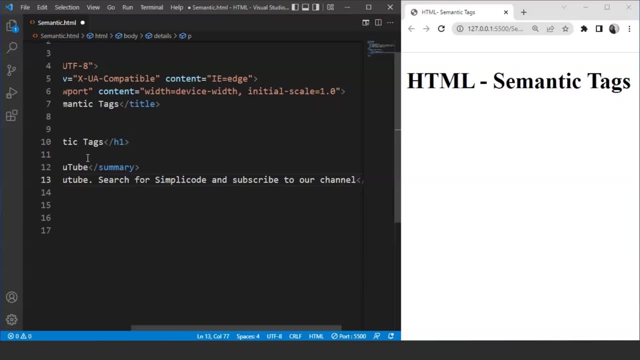 It means we are providing any details within this particular tag. So let's check the output now. Let's check the output, Save the program And you can see here we have the text present inside the summary tag, So we have YouTube written over here. 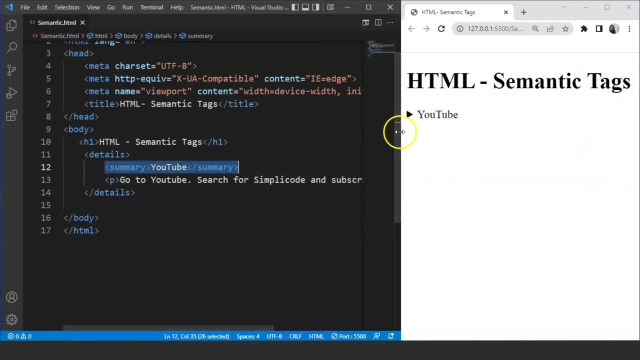 We can see here. we have used the word YouTube inside the summary tag, So we have YouTube written over here. Now you can see we have this arrow shaped thing over here. Before YouTube. we have this arrow shaped thing. Click on it and see it expand. 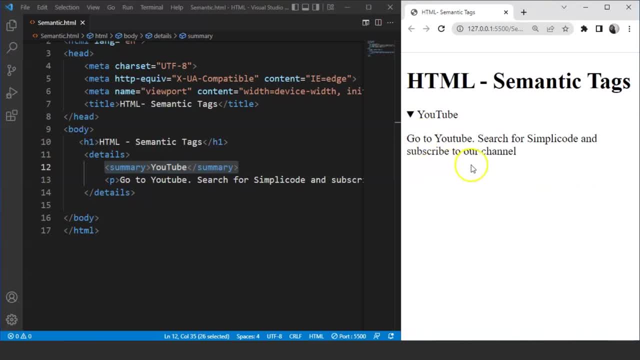 Now we have this paragraph over here. Fine, It says: go to YouTube, Search for Simply Code and subscribe to our channel. We can also increase the size of the text. Now we have this paragraph over here, We can also increase the size of this paragraph. 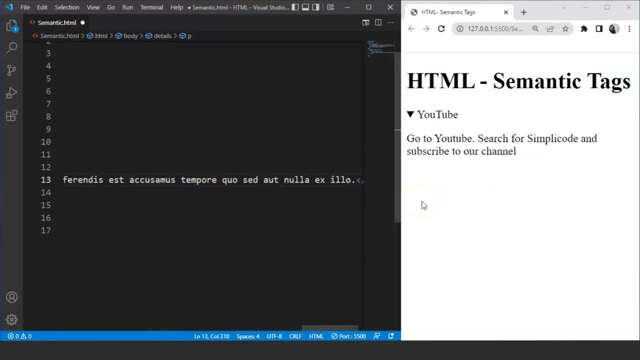 Let's do one thing over here. We'll write over here: lorem 35.. We are going to use 35 words from this paragraph. Save it now, Open it again And here you can see we have this whole paragraph present over here. 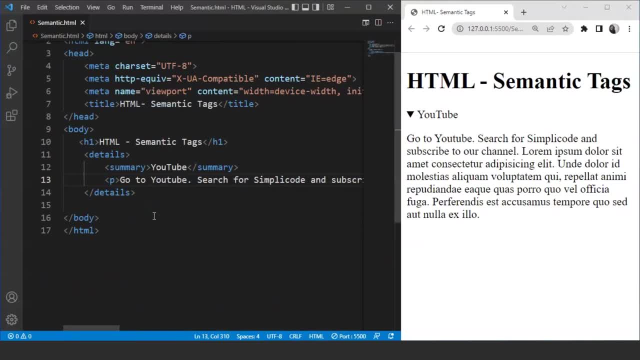 Fine. So it's working totally fine. But other things we can do is we can remove this paragraph from here And just do one thing: Just remove this summary as well. So we'll remove this summary as well. Now save the program. 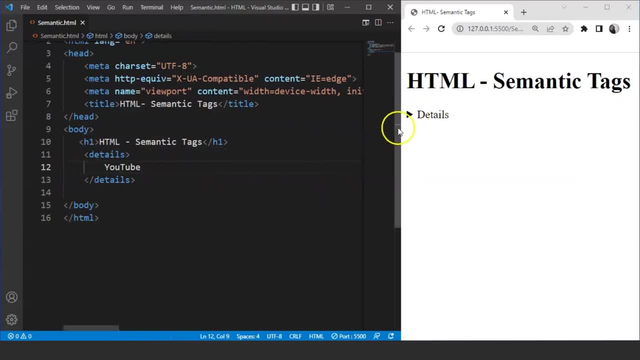 And you can see. we have details written over here by default. This is the tag name. Click on it and you can see. it says YouTube. Fine, So it's totally fine if we are not using the summary tag or the paragraph tag inside the. 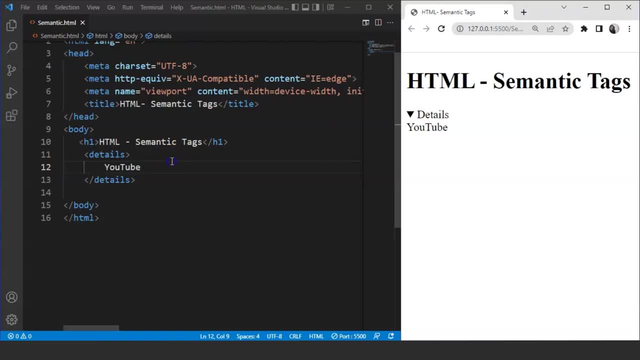 details element. It's totally up to us what we want to do, So let's just undo what we did till now. Now, another thing we can do is we can style these elements according to our need. So let's say, we are going to style a paragraph with the font color as red.